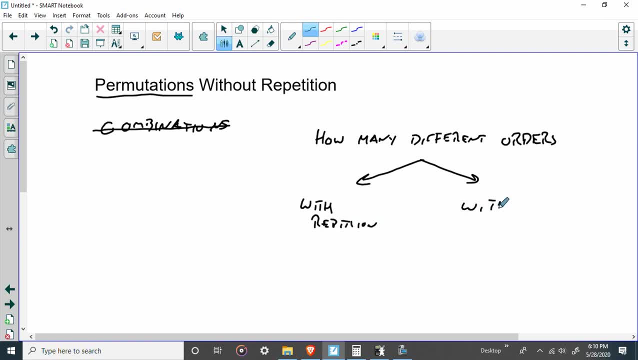 And without Now, when you think, with repetition, if I said, hey, your pin number right, Pin right, We shouldn't have to actually say personal identification numbers. When you say pin number, it's actually your personal identification number number, Silly, But pin number is typically four digits, right. It can be up to six, but it's a four-digit number, right. 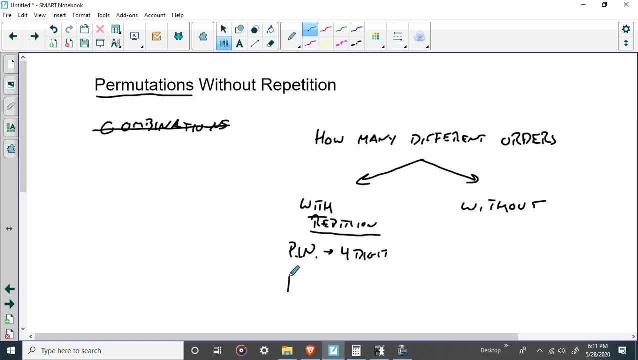 And you use it at the bank, right. You swipe your card, okay, And you could say, hey, I need. I have a first slot, a second slot, a third slot and a fourth slot, okay, And pretty much what you have is you have 10 numbers to choose for the first one, right. You have 0,, 1,, 2,, 3,, 4,, 5,, 6,, 7,, 8, and 9,, right. You have the 10 single digits. So you have 10 here, 10 here, 10 here and 10 here, right. So all you'd say is this is: I have 10 to the fourth power. 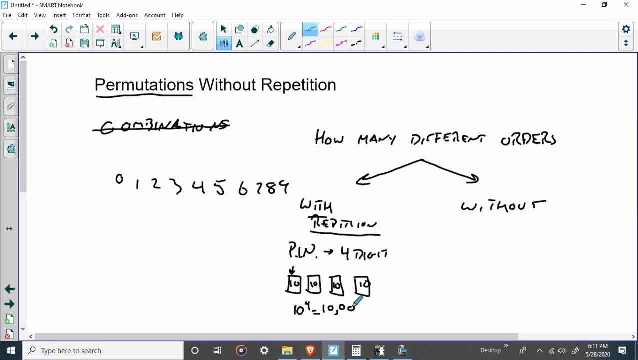 And what does that mean? That you have 10,000 different pins that you could make. okay, Now, without repetition. we'd say something like this: You can't use the same number twice right? So that becomes a different thing, okay. So if I said, say, for example, you're running a race, right? 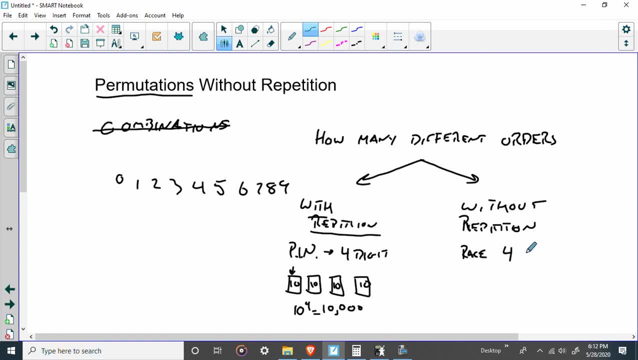 You have four people racing, right. How many different orders can they come in right If you have four people racing? somebody's coming first, somebody's coming second, somebody's coming third, somebody's coming in fourth? Well, again, you have four slots, And let's think about this: How many different people could finish first is four, But once someone's finished first, they can't also finish second, So you only have three people left to finish second. Once you have that, two people and one. 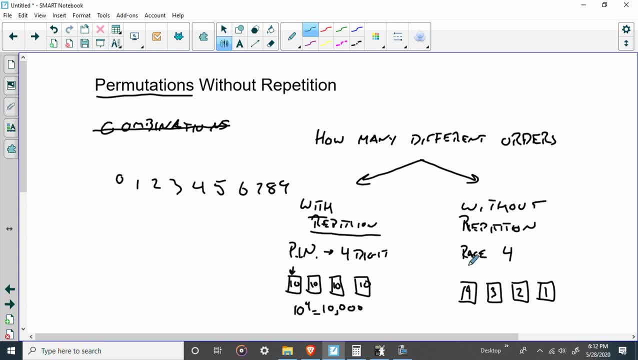 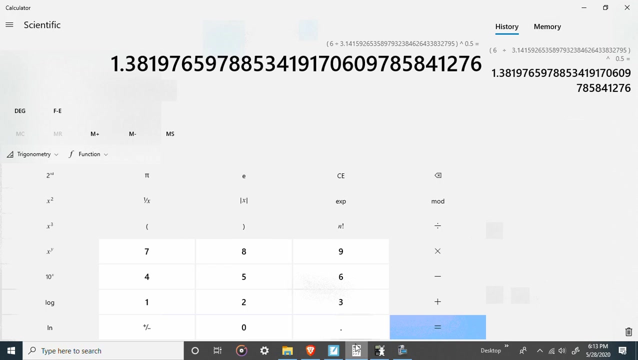 What does this become? Four times three times two times one. So you can't be. there's no repetition. You can't come in first place and second place. You can't come in second place and fourth place, And this is what we talked about, And this would be four. factorial right, Which we said other day, was four times three times two times one. So four times three is 12.. 12 times two is 24.. 24 times one is 24.. And I told you guys, if you have a calculator, it's the exclamation point, So it's right here. So I'm going to clear this. 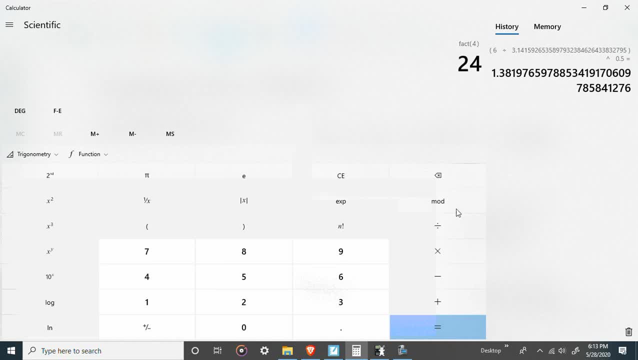 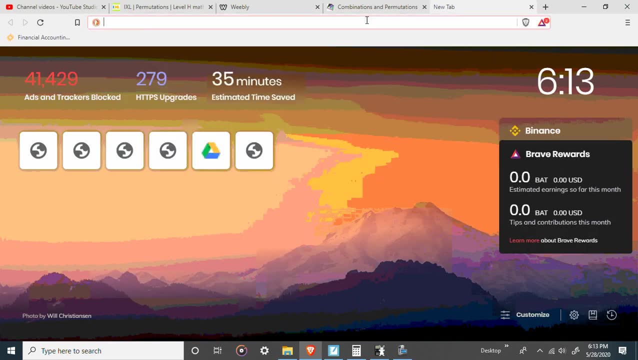 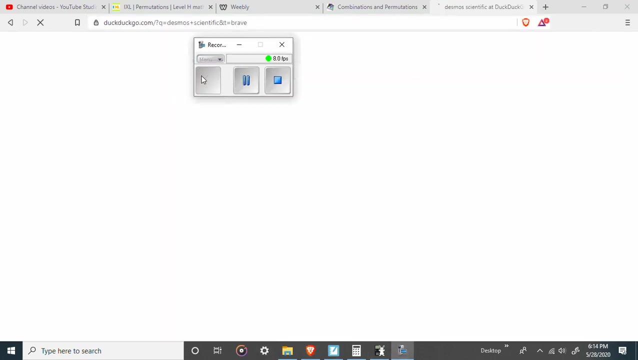 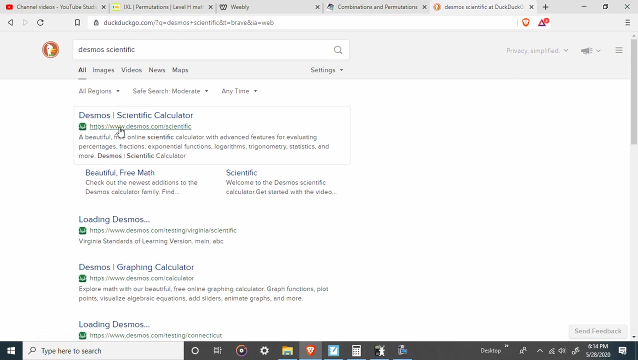 If I said what's four factorial, it will tell me that it's 24.. I'm on Desmos. If you guys are on Desmos, I'll keep that open. Okay, Sorry about that. If you don't have a calculator at home, you don't want to use your phone. If you go to Desmos, just type in Desmos Scientific and you can have a calculator and it's under the function. 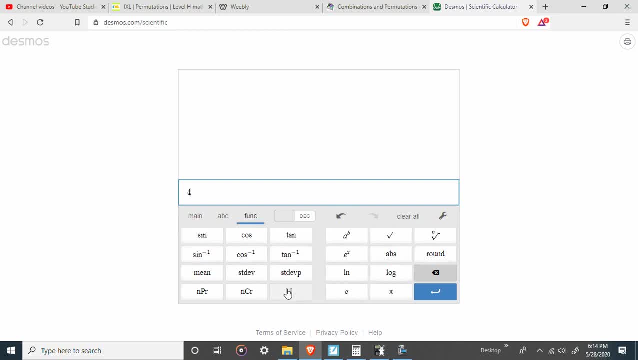 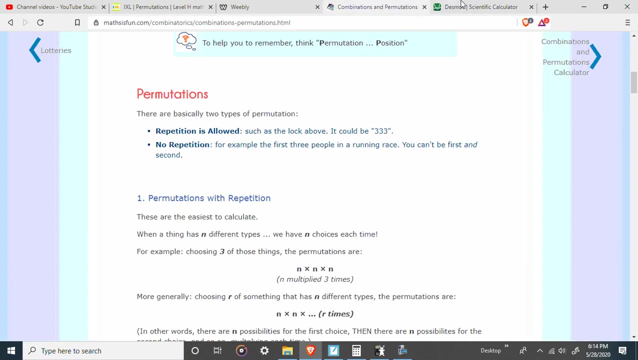 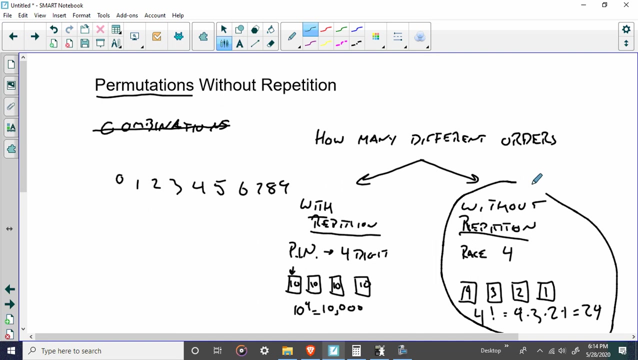 So if I said four function and you're looking for the exclamation point, You can also just type it on your keyboard. So if I said four and I type in shift and one, it will tell me that it's 24.. Okay So let's take a look at some of the questions you might be asked. They're really pretty straightforward. We are only going to be talking about without repetition problems today. Okay So I'm not a huge fan of IXL because they just lump these as permutations and they don't talk about repetitions. 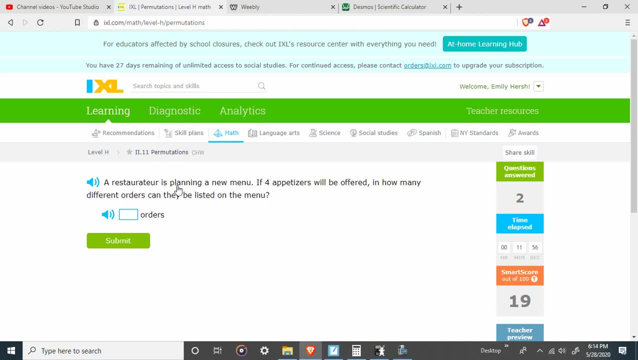 Okay. So I'm not a huge fan of IXL, because they just lump these as permutations and they don't talk about repetitions, repetition, not repetition. but another day, okay. so again, a restaurateur is planning a new menu. if four appetizers are offered, how many different orders can they be listed on the menu? again, you, 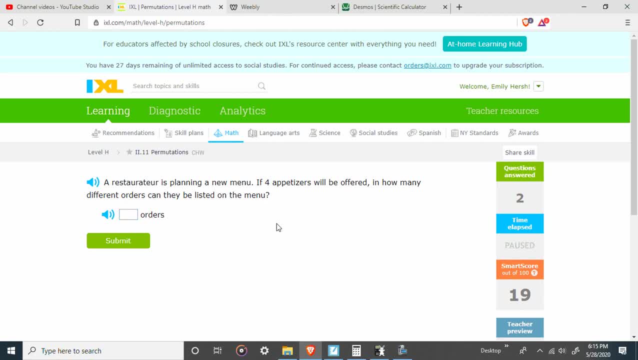 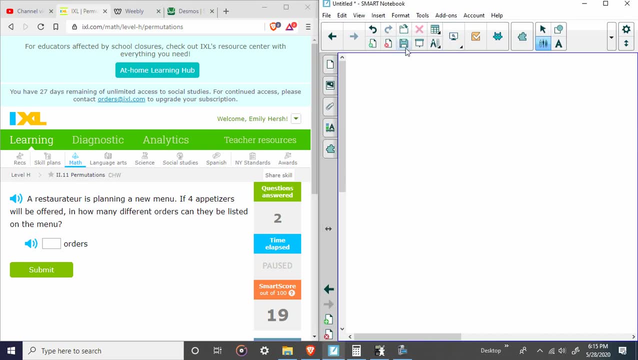 you're gonna have four for the first one, right four. i can't write on the screen, hold on. you're gonna have right four for the first slot, then three, then two, then one. so this would be four factorial. so four factorial, we already know, is 20. okay, says laura, and her friends are trying a. 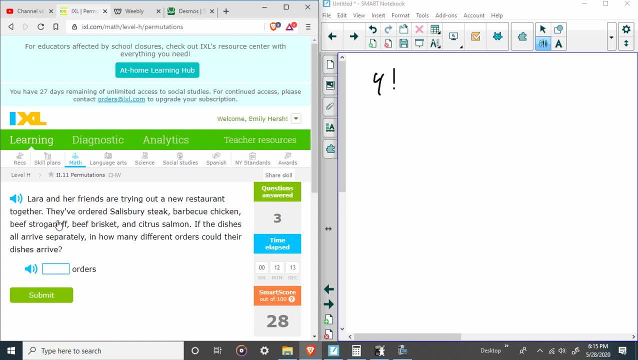 new restaurant together. they've ordered salisbury steak, barbecue chicken, beef stroganoff- ah love beef stroganoff, beef brisket and citrus salmon. um, no vegetarian orders. all right, i have the dishes all arrived separately. and how many different orders could dishes arrive well? 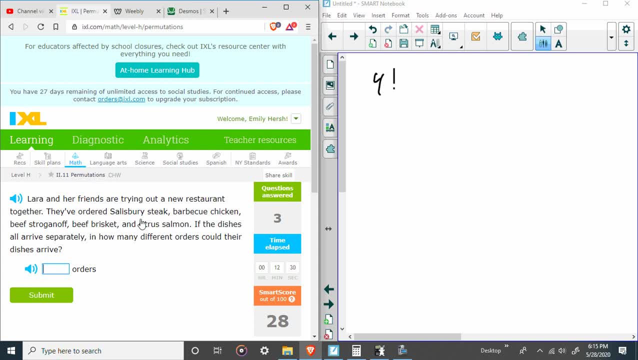 you got salisbury steak, barbecue chicken, three, four, five different dishes here, right? so again same thing. one comes first, then there's four left to come second and three left to come third and two left and one left. so five times four times three times two times one, um, so again, five times four is 20. 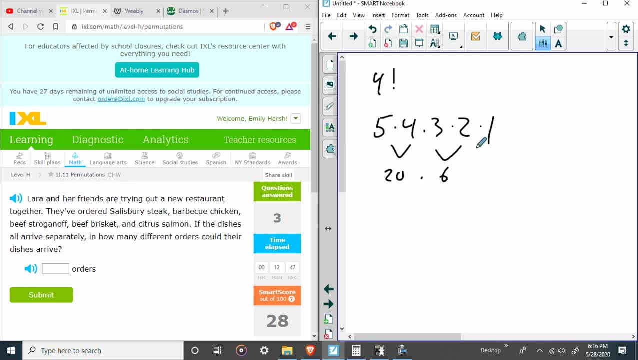 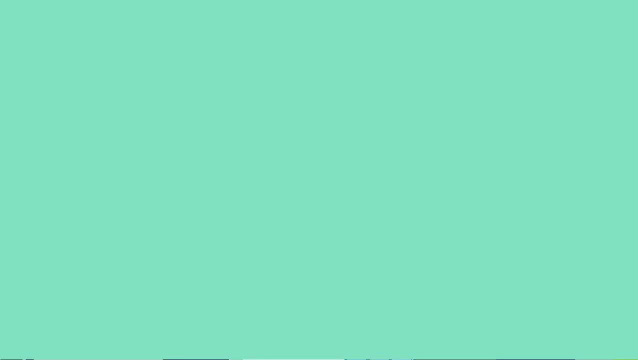 uh, three times two is six. uh, 21 is just times one, doesn't really matter. 20 times six is 120. so there's 120 different orders and you'll see these numbers get really big really fast. so, um again, if you have a calculator handy, you just go and you type in five factorial right, five dishes. 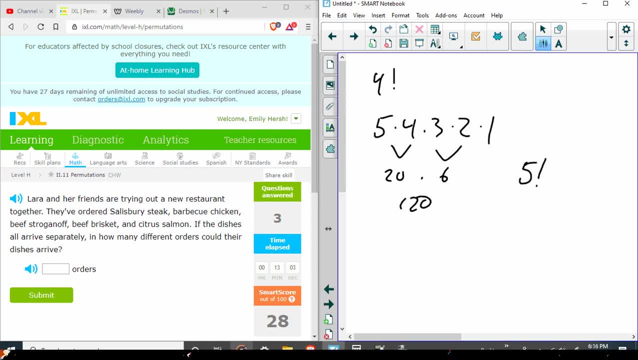 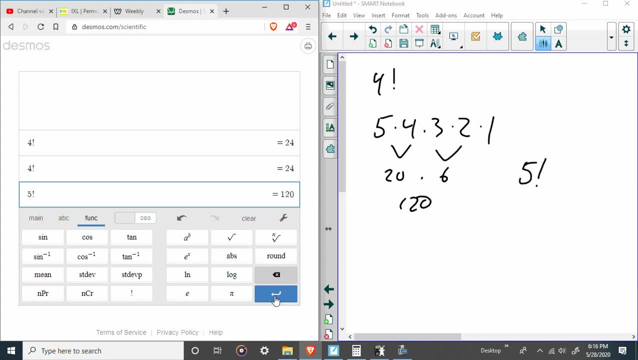 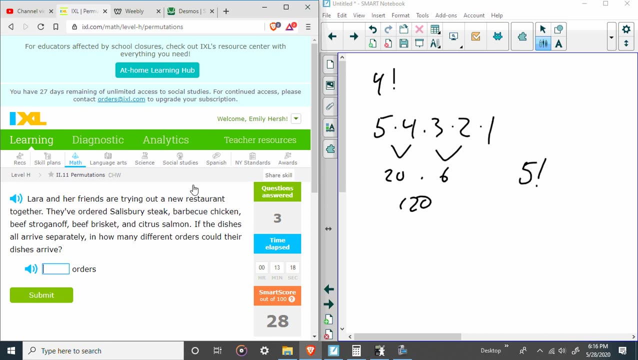 how many ways can they come out? so you go out there, you go wham, you break out your calculator, you say five factorial and it will tell you that it's 120. i hope you guys can hear that bird screeching in the background, by the way. um, all right, so again. well, yeah, you got 120 different orders over there. 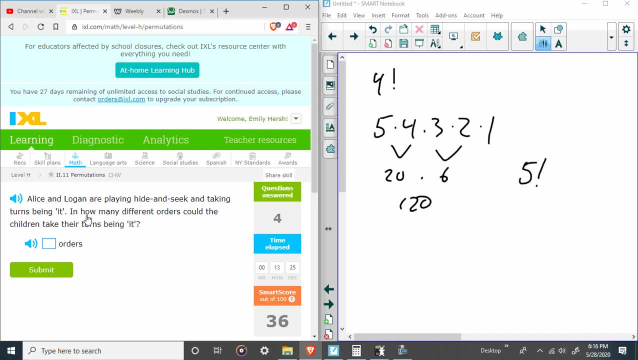 all right. so alice and logan are playing hide and seek and taking turns being it. how many different orders could the children take turns being it? well, i hate, say, but hide and seek with two people is pretty. oh, that's a rough one, i tell you. so that's just two people, right, and two factorial is two times. 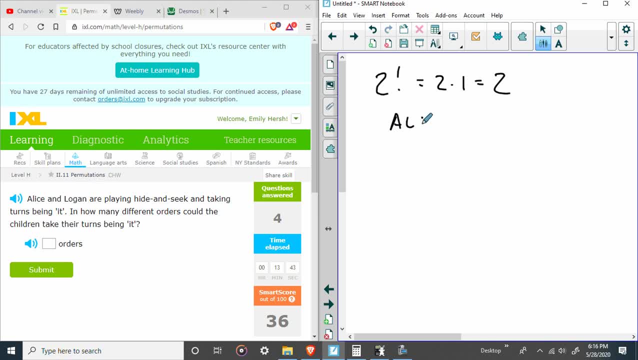 one, which is just two right, in other words, alice then logan- that's one way, right. or logan then alice, right, that's, that's the other way. there's only two different ways that this can happen. okay, um, but you guys should be surprised: the faster this um, the bigger these numbers get um. 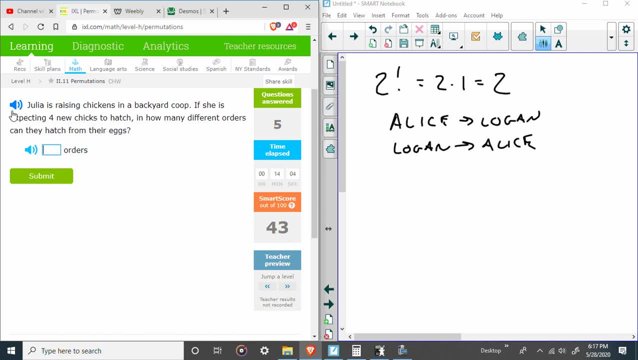 the bigger these numbers get, the higher the 여운 too will grow. just huge numbers very quick, to the point that if you have something like 10 factorial, it's just such a gigantic number. okay, julia's raising chickens in the backyard coops if she's expecting four new chicks to hash in. how many different? 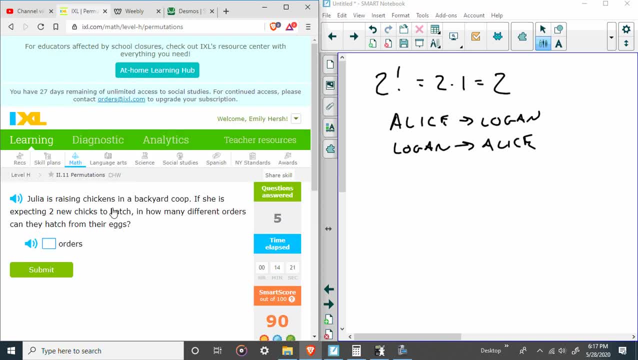 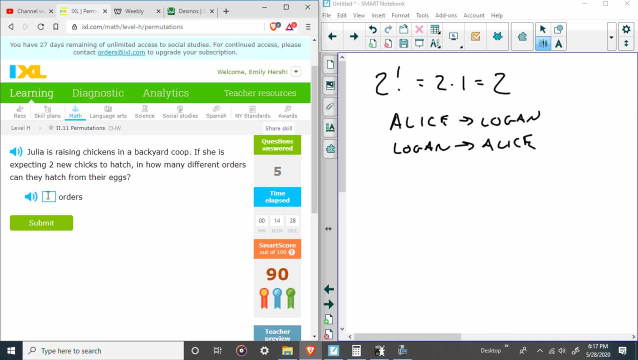 orders. can they have their eggs again for factory? let's, let's skip up levels. oh, we're entering the challenge zone, oh god, okay. so same question. so pretty much what you're looking for is there's going to be no repetition. two, two new eggs to hatch. 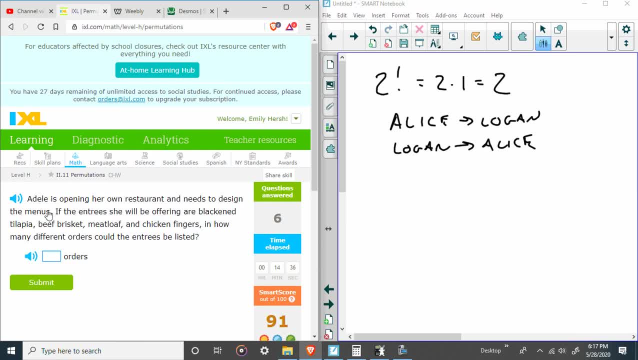 Adele. Oh, it's Adele. She sings songs about love and loss. She's opening her own restaurant and she needs to design the menus. If the entrees will be offered are blackened tilapia, beef brisket, meatloaf and chicken fingers. 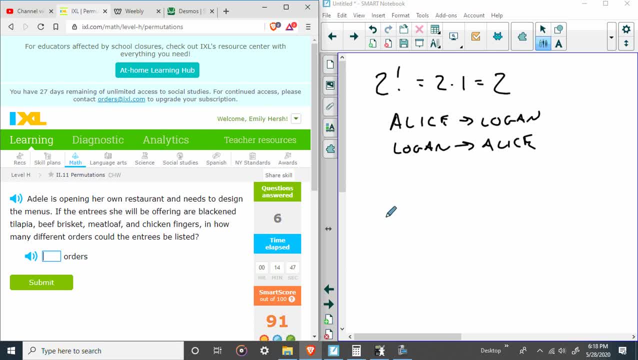 Again, no vegetarian option, And how many different orders could maybe be listed. What do you got? You got four dishes, four factorial. What do we say? That's going to be 24, right? So again, there's only so many numbers I can ask you, because there's only so many numbers you can get, okay. 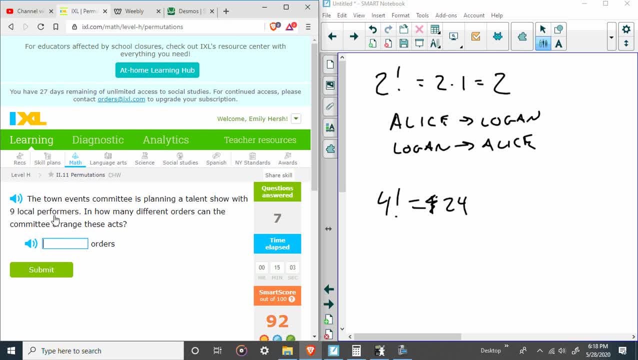 A town events committee is planning a talent show with nine local performers. And how many different orders can the committees be arranged? And can the committee – how many different orders can the committee arrange these at? So again, so nine factorial, Nine factorial you're going to see turns into a very big number, very, very quick. 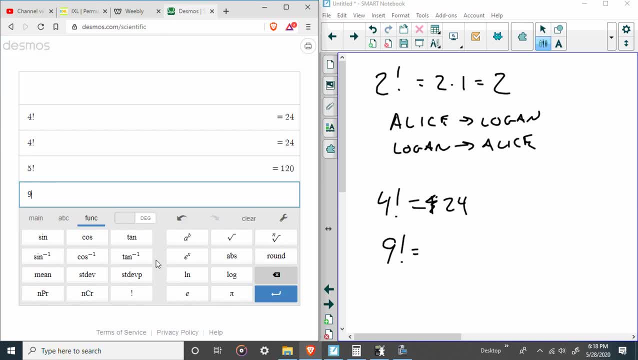 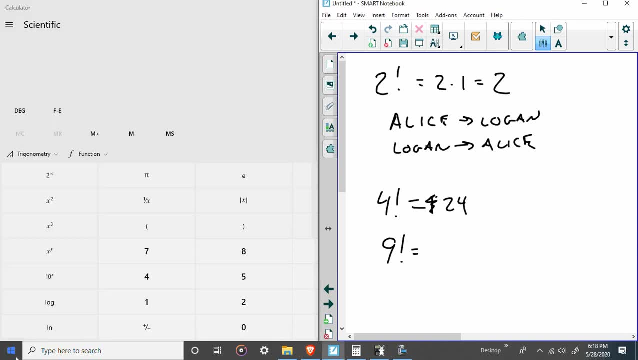 So again you break out your calculator, You say, hey, what is nine factorial? And you find out that there's 362,880 different ways. okay, So again these numbers get real, big, real fast, And you wouldn't think that right. 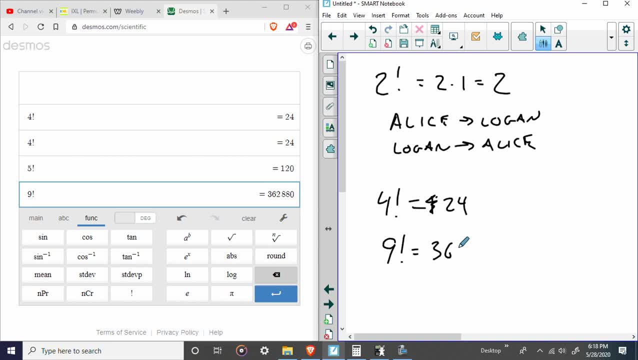 That's only nine different musical acts And you could arrange them 362,880 different ways, Like, wow, that's a lot for just nine different acts, right. So think about that: You got your nine favorite acts, right. 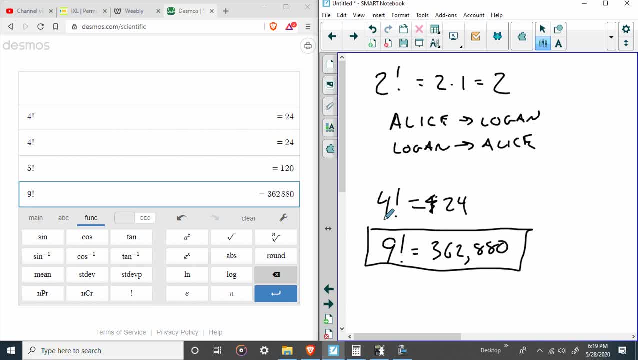 You got whoever you like out there, And if you were having an all-star concert, how many different ways could you organize them? Insanely enough, there's 362,880 different ways. you can just arrange those nine groups And I know that sounds –. 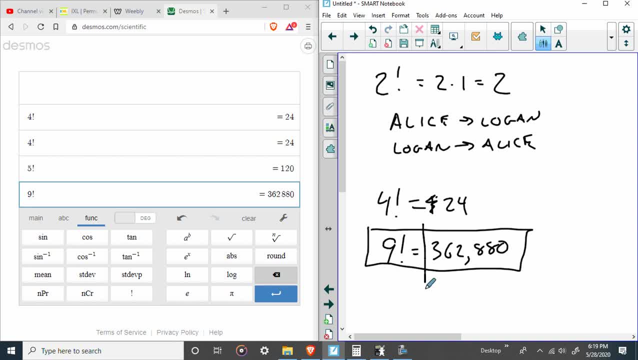 I know that sounds crazy, but that is true. okay, You can even try it sometimes if you have a ton of free time on your hands to write out 362,000 different ways, okay, So I'll find you guys some more complicated ones for Monday, and we'll talk about it more on Tuesday. Thanks guys, Bye.